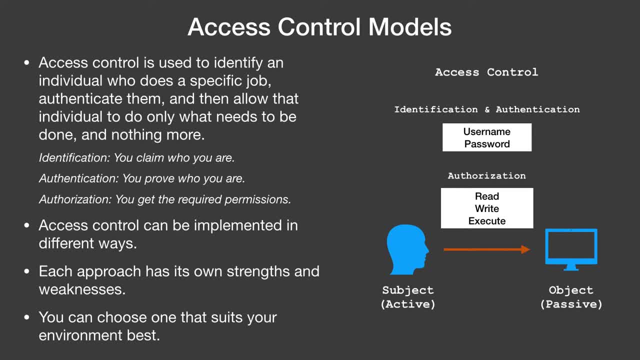 one more important thing. As you are looking on the right side, there is a subject and there is an object. A subject is an active entity that is trying to access something, say a file. Here the user is subject. Subject is an active entity that is trying to access something, say a file. Here the user is subject. 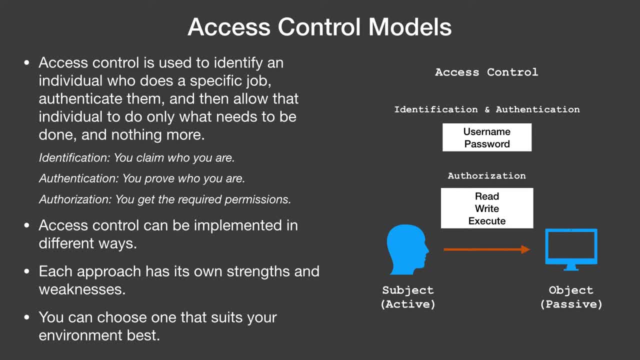 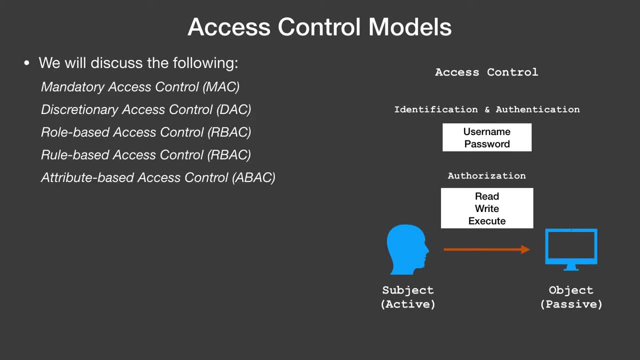 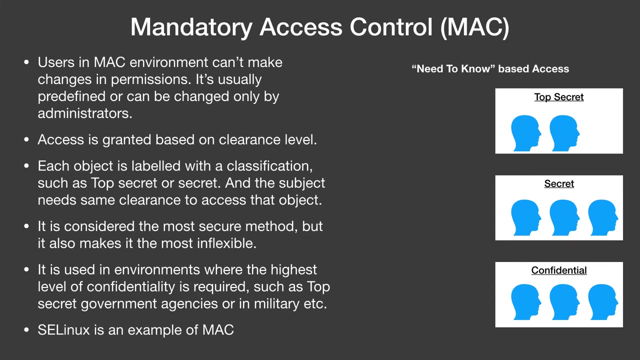 Subject is an active entity that is trying to access something, say a file. Here the user is subject: The active entity and the file is object: a passive entity. Now I'll discuss the following access control models in detail. Mandatory access control model MAC. This model is very restrictive, You won't see. 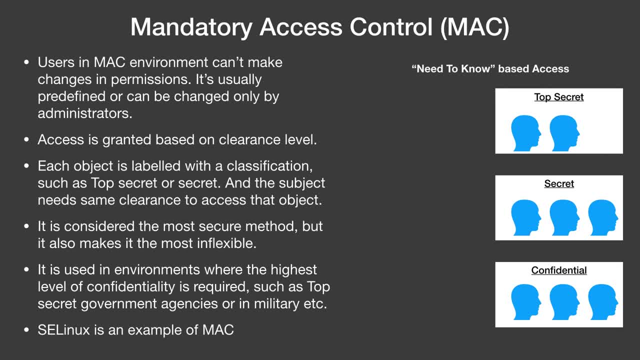 it. in common environments. The subjects are labeled with different classifications, such as top-secret or confidential, and the only subjects having the right security clearance can access an object. Users in MAC environment can make changes and permissions. It's usually predefined or can be changed only by administrators. 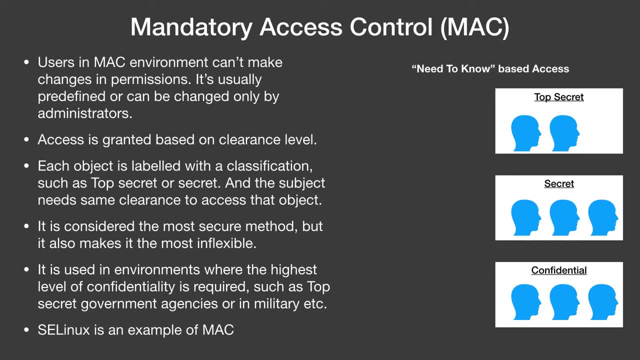 Access is granted based on security clearance level. It is considered the most secure and most inflexible access control model. It is used in many ways to used for highest level of confidentiality, such as in government agencies or military etc. I say Linux is an example of Mac implementation. 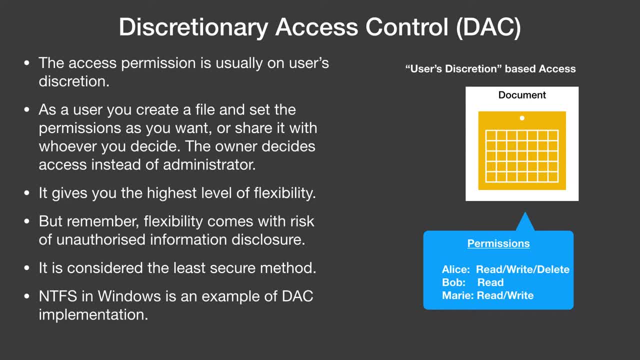 Discretionary access control. in this model, the access permission depends on users discretion and that's why it is named as discretionary access control. let's say you created a file and set the permissions as you want it and shared it with others, all without asking your administrator or anyone else, just like. 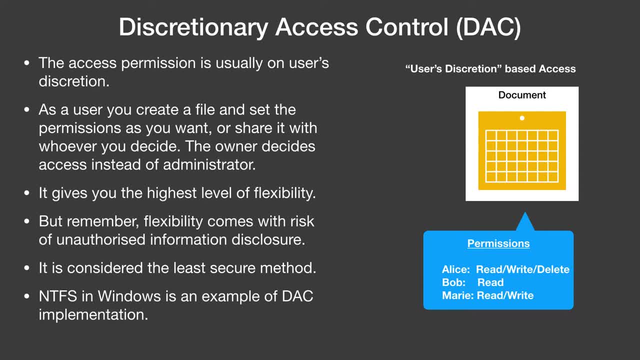 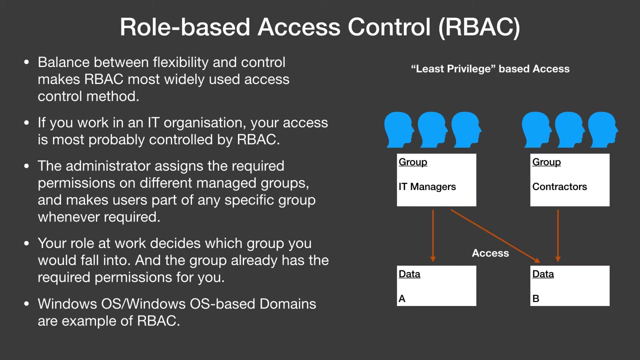 that it gives you the highest level of flexibility. but remember the flexibility here comes with risk of unauthorized information disclosure, so it is considered the least secure access control model and TFS in Windows is an example of DAC implementation. role-based access control are big. role-based access control is balanced. 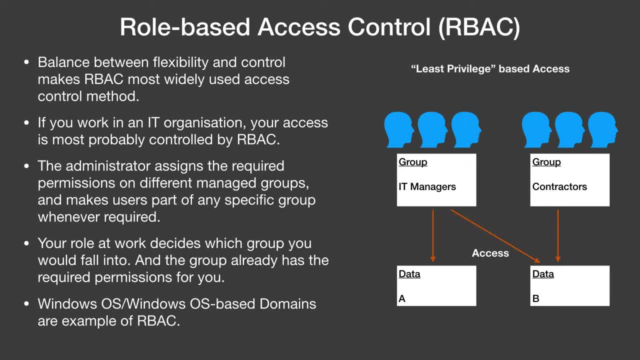 between flexibility and control, and that's what makes it most widely used, especially in organizations or in large network environments. neither the access is controlled completely by users, such as in DAP, nor by administrators at a granular level, such as in Mac. it is done in the 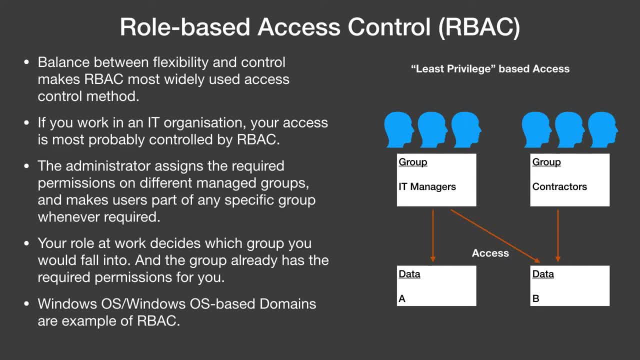 middle of both, the administrator creates groups based on job roles and responsibilities and assigns the required permissions onto those groups. whenever new individual comes in, the administrator will just make that individual part of the required group according to the job role, and if someone moves from one role to another, the admin will just remove them from the previous. 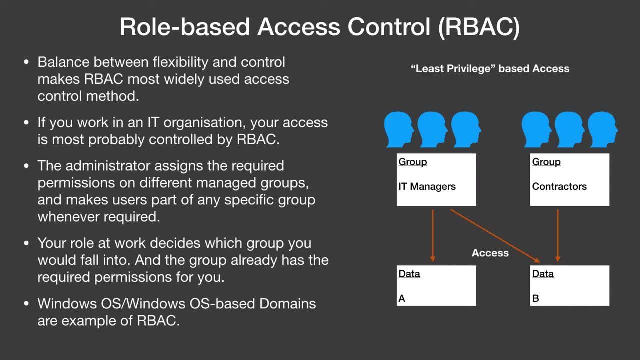 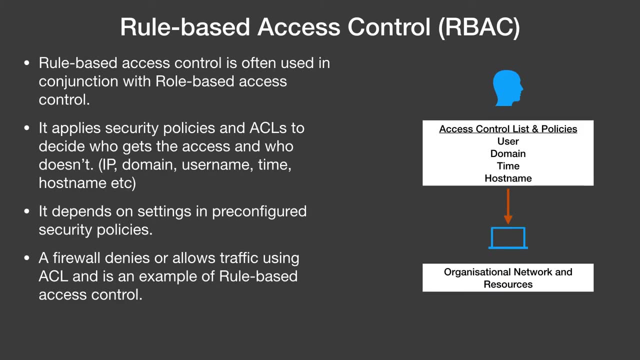 group and make them the part of the newly assigned group assigned one and if they leave, the access will be removed accordingly. Windows or Windows based domains are common example of RBAC Rule-based access control. another RBAC Rule-based access control is often used. 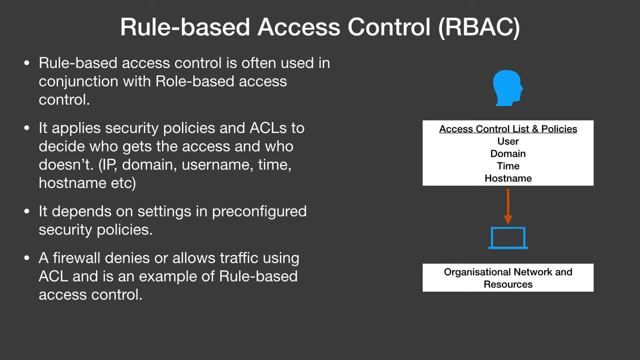 in conjunction with role-based access control. It applies security policies and ACLs to decide who gets the access and who doesn't. The ACLs could be based on internet protocol, address, domains, usernames, timing, hostname and etc. It depends on settings and pre-configured security policies. A firewall denies or 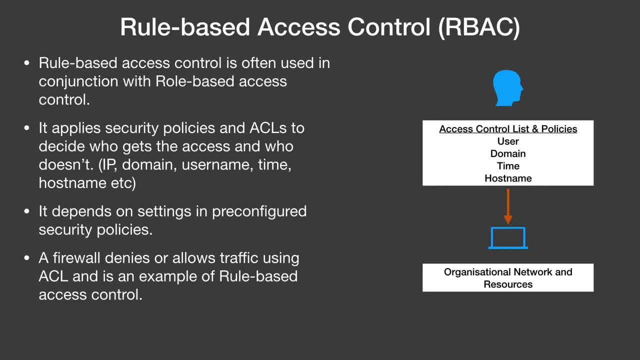 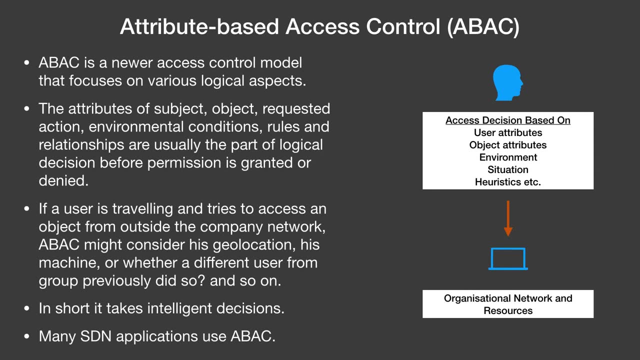 allows a security policy to be used. A firewall denies or allows a security policy to be used. A firewall denies or allows traffic using ACL and is an example of rule-based access control. Attribute-based access control, or ABAC. ABAC is a newer access control model. 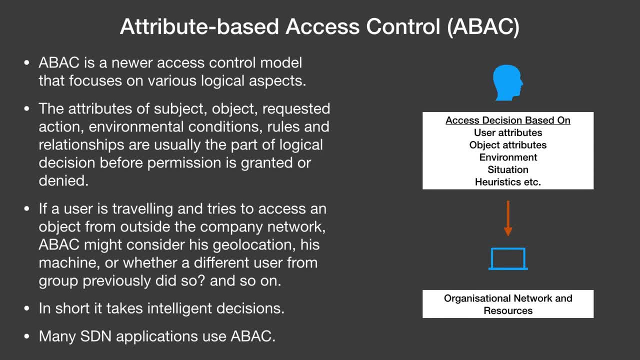 that focuses on various logical aspects: The attributes of subject, object, requested action, environmental conditions, rules and relationships are usually the part of logical decision before permission is granted or denied data. but in case of ABAC it will be looking at user characteristics data.